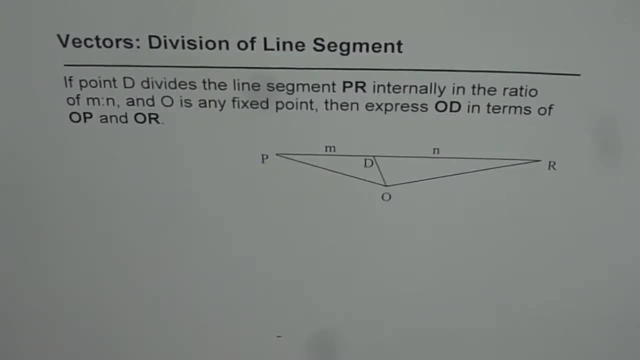 Vectors: Division of line segment. It's a very important topic and in this example we are going to derive a general formula so that we can divide a line into a fixed ratio. Now that division could be internal or external. This particular video is for internal, but we will kind of extend it for 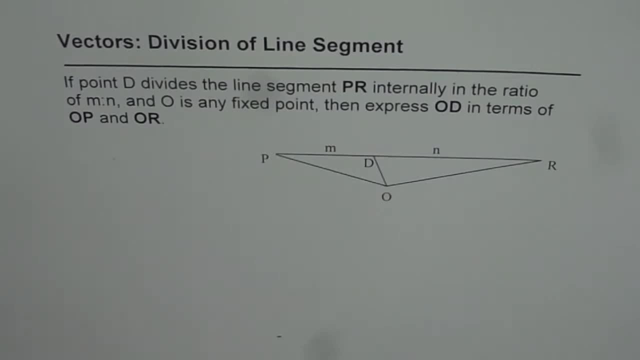 external division of the segment. also, The question here is if point D divides the line segment PR internally in the ratio of M is to N and O. is any fixed point then express OD in terms of OP and OR? Let's have a good look at the sketch which is given here. P and R are the two given. 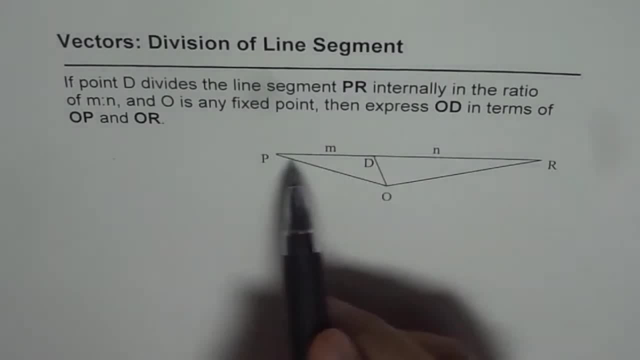 points. We know them right. We need to find a point D in between P and R which divides PR in the ratio of M to N, right? So that is the question, And we need to express OD in terms of OP and OR. Now, let's do it Now, as you can see from here what. 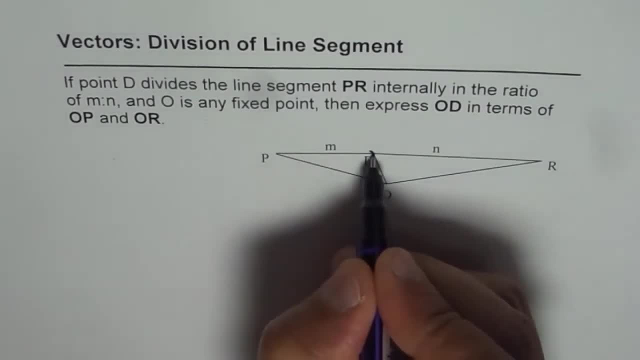 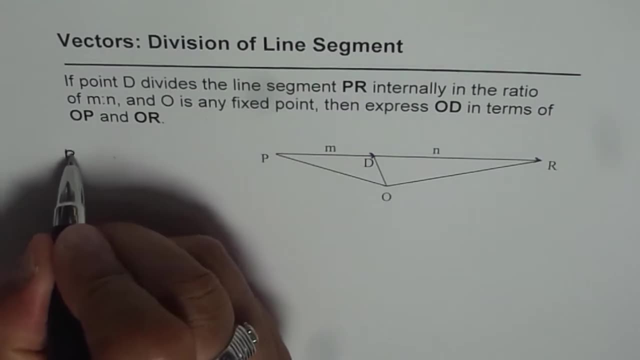 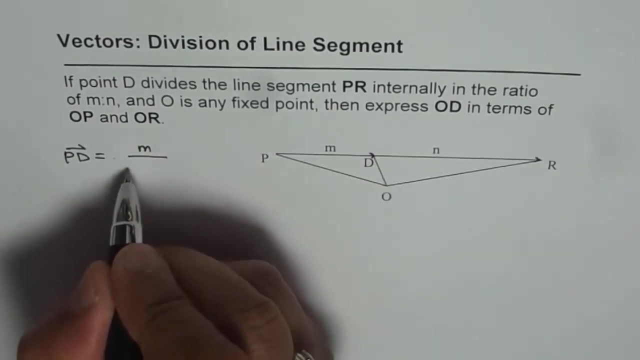 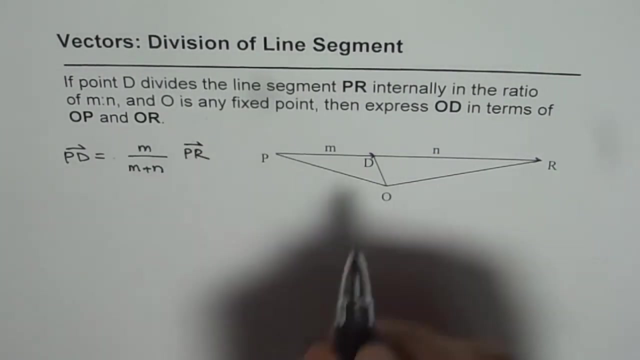 we can do is we can write what PD is in terms of PR. Now PD vector: PD is equals to M divisions out of total M plus N. So that is the scalar multiple of PR, right? So these are collinear vectors and therefore PD is a scalar. 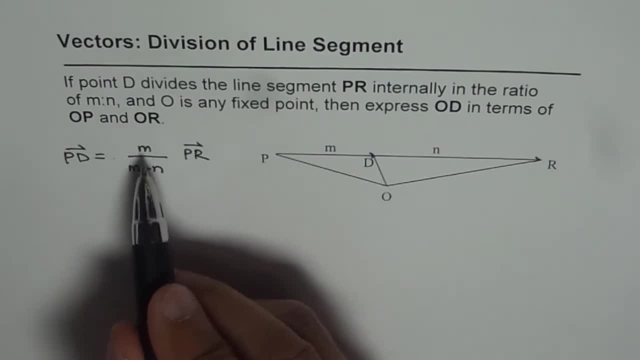 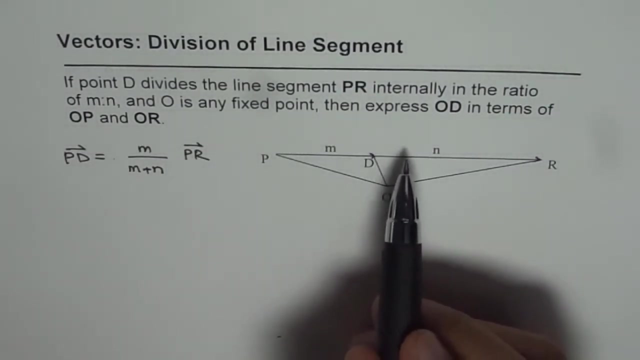 multiple of PR and the ratio is M over M plus N. So that is the scalar multiple. So that is how we get the relation between PD and PR. Now we will try to relate PD and PR with OD, since we want to express the relation between OD and OP and OR. 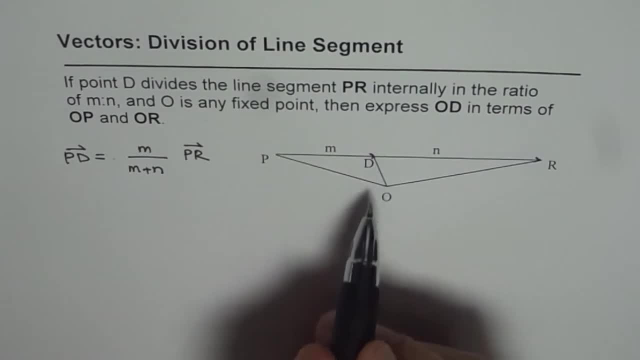 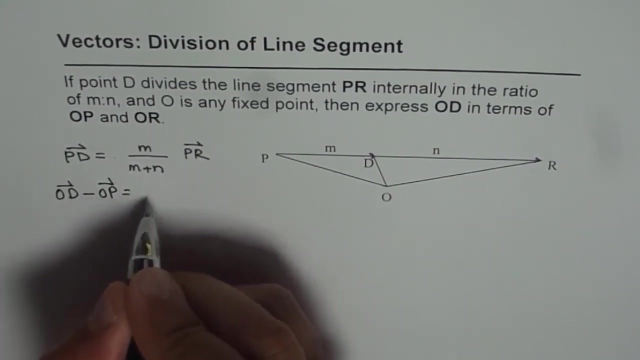 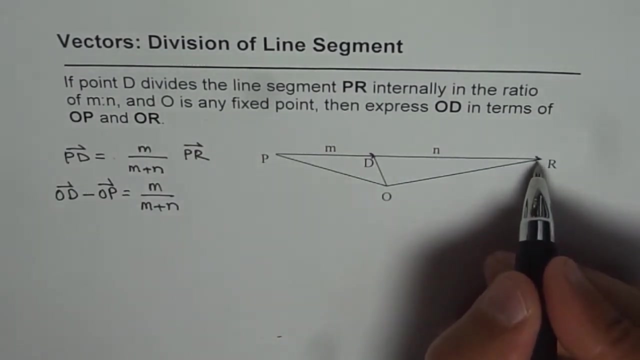 Now PD in terms of OD will be what? So P to D will be OD minus OP, correct? So we can write PD as OD minus OP and that is equals to M over M plus N. What is PR? PR is OR minus OP, right. 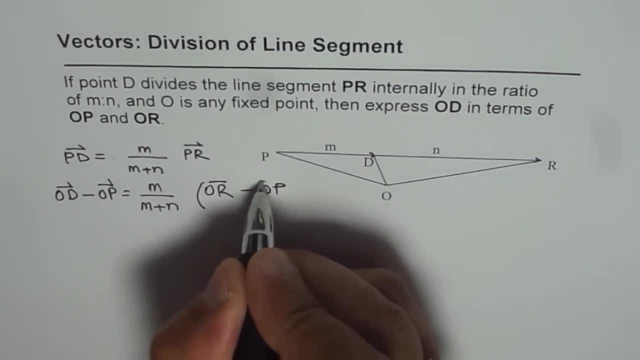 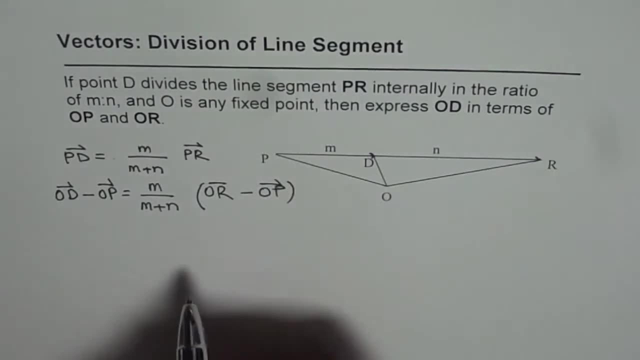 So the vector terminates, initiates from P, terminates at R and therefore it is OR minus OP. Now, what do we need to find? We need to find OD right. So let's isolate OD from here. OD is equals to, and expand this, We get M times OR right. 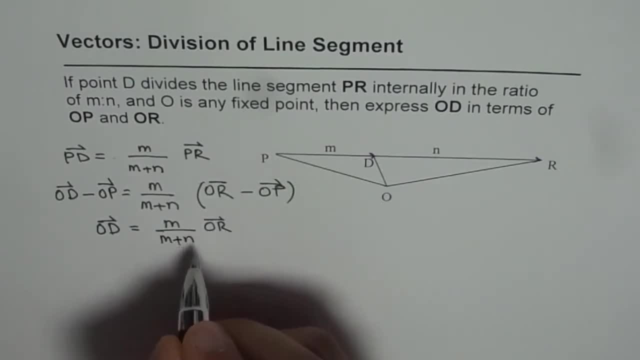 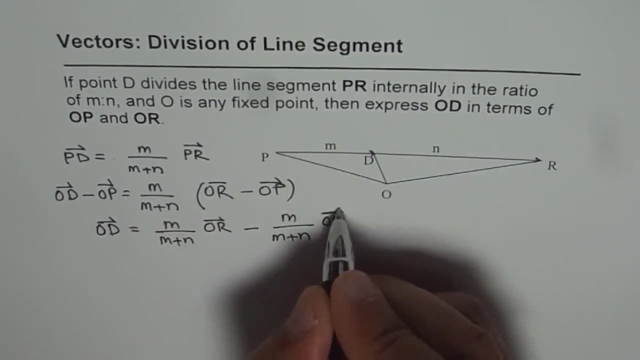 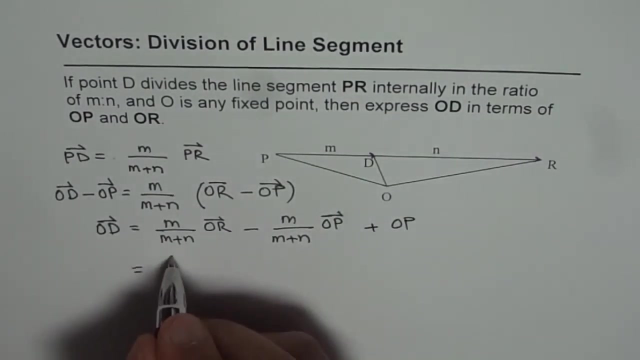 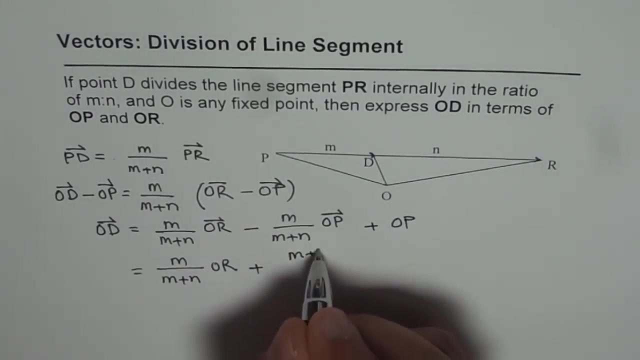 M over M minus OP. M over M plus N, OP plus OP right plus OP correct. Now let's simplify this part. We get M over M plus N, OR. Now here it is. if I take M plus N, the numerator will be: let me write plus first, M plus N times OP, which is M plus N minus N. 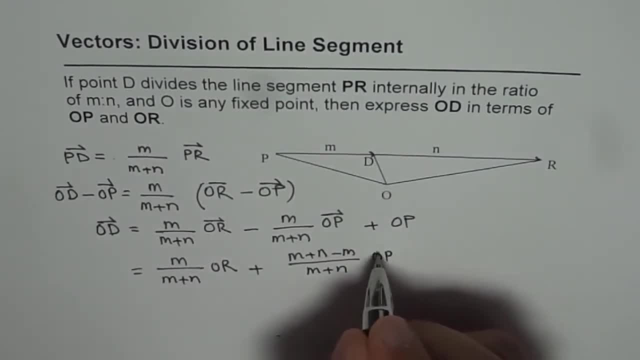 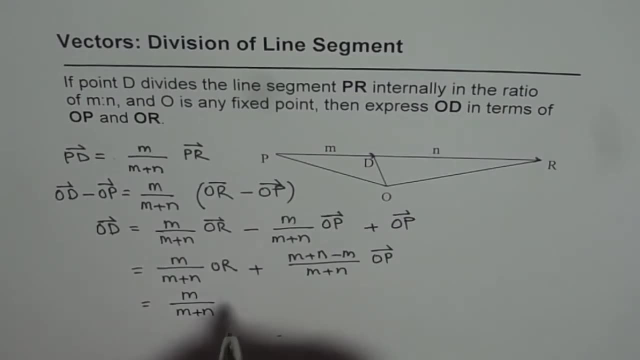 So from here we will have OD over AB and now enter ourения. So the is our veterinarian going to stop APP? So excellent, Now, this is it. Now, here we have OD, So for ourẻ is it right. OK, So that's it. 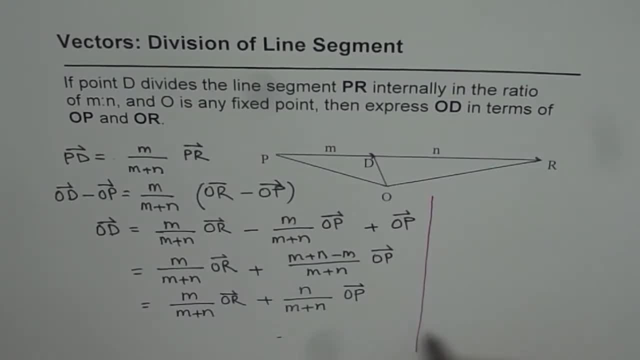 OK, so now application in vectors, and therefore we should always, you know, highlight it. let's say: OD for us is equals to M over M plus N, OR plus N over M plus N, OP. now, in a given scenario, O could be the origin right in that case, OR OP and OD. 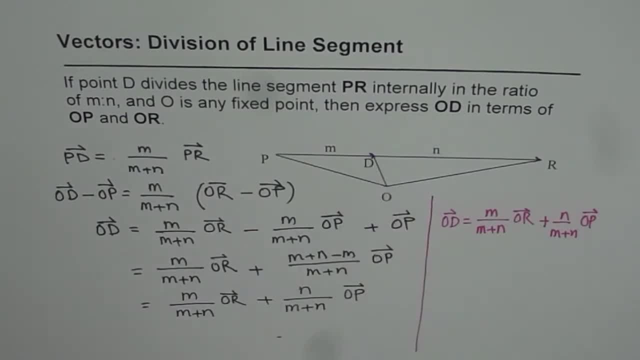 becomes position vectors and therefore we can find the coordinates of point D, which divides the line segment internally. right now, as an exercise, what you can do is we can do external division. external division really means that we are given a vector P&R right and we are going to divide with point D, which is outside in the